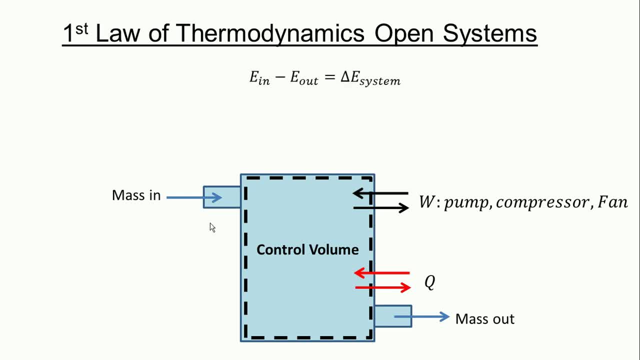 To describe open systems, we apply the following concepts: Basically, the energy in minus the energy out equals the change in energy of the system. This equation can be expanded to describe the open system below. as shown in the figure, An open system energy transfer occurs in three forms: in terms of heat, work and mass. So these are the three things you've got to drill into your head to become a master. 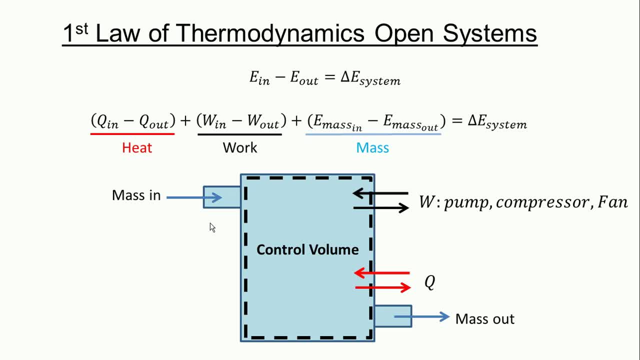 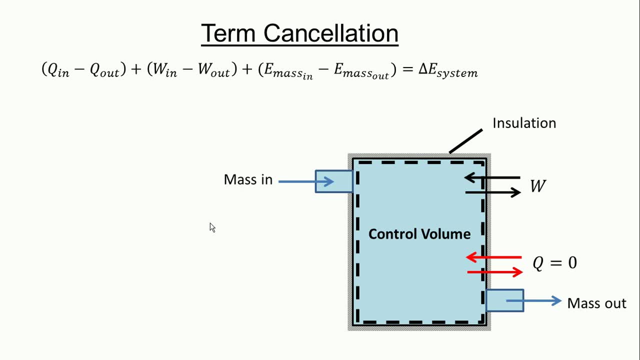 chefs. It's there for thisıy. Now that we kind of know the basic terms that go into An open system, See how these terms come into play and how you can Simplify your analysis to describe an open the system Models. So the figure shows the control volume. 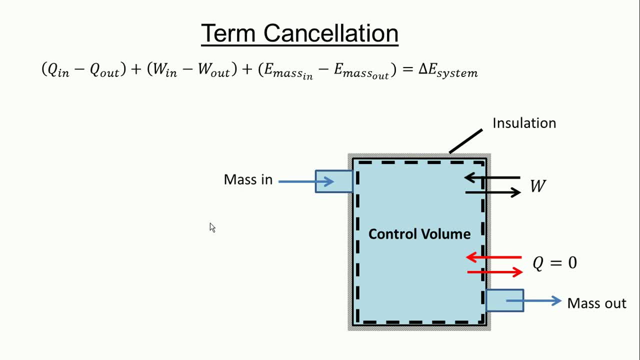 Or in open systems. Okay, Usually we can serve this. This Sort of You could say would be US. So let's start this country Stop Auf. an adiabatic process. That basically means there's no heat transfer between the system and the surroundings, and we can then collect the heat term Further if you don't have. 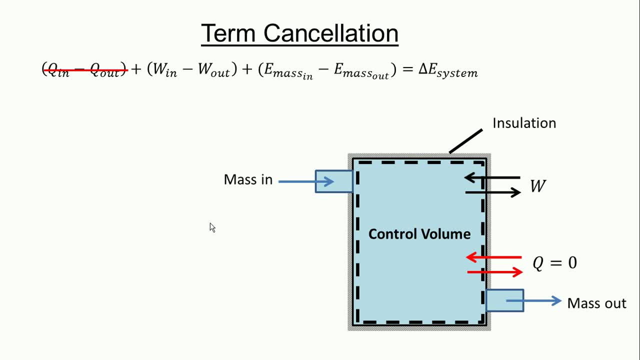 a rotary device that is supplying energy to the system or the system is not turning a rotary device to supply energy out of the system, we set the work term equal to zero And if your system is in steady state, the term on the right-hand side is set equal to. 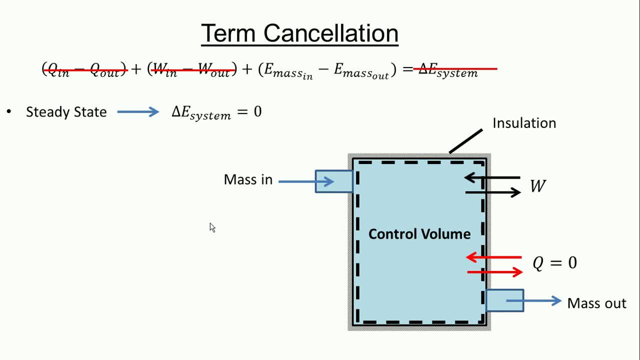 zero and in many engineering calculations this term has to be set equal to zero to perform hand calculations. Otherwise, if it's not equal to zero, then you'll have to apply numerical methods to get the answer. And lastly, the energy transfer by mass. that expands out to include more terms such as: 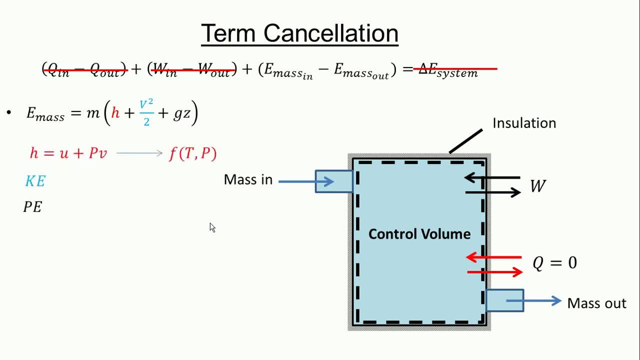 enthalpy kinetic energy and potential energy. So enthalpy basically contains within it the internal energy and the flow work of the system, and this is a function of temperature and pressure. So if you temperature Pressure changes between the inlet and the outlet, this term is going to show up. So